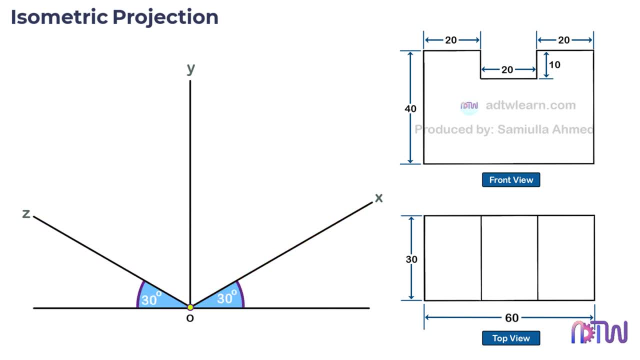 We can see the x and z-axis are inclined at 30 degrees and the y-axis is at 90 degrees. These axes are called the isometric axis. Now we can draw the isometric view on this axis. Before drawing, an important thing which we have to remember is that when we draw the 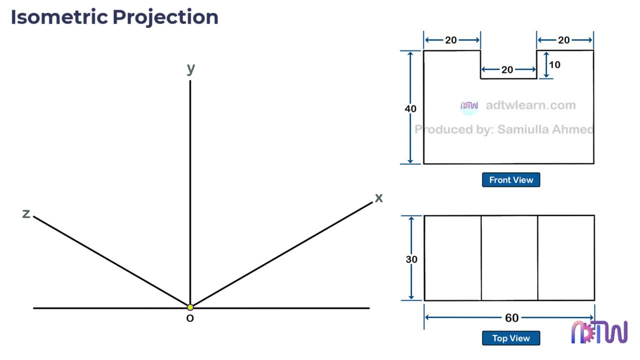 three-dimensional view of the object. the maximum edges of the object should be visible. For example, consider this object. If we look at this object from this angle, we can see only a few edges. If we rotate this object and look at this from this: 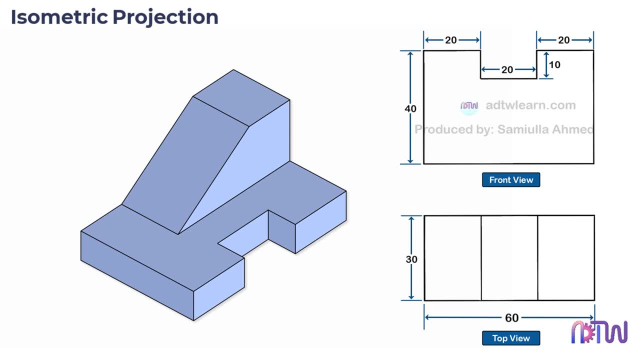 angle we can see more details. Therefore, we need to carefully select whether to draw the front view of the object facing on the x-y plane or y-z plane. Consider this given figure. By looking at these two views, you need to imagine the object. When you see this object from the front, 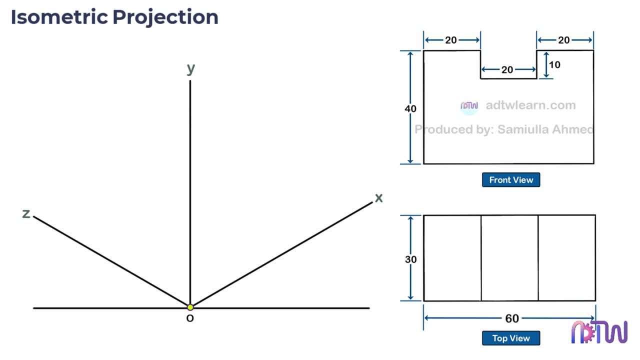 this is how it looks. and when you see it from the top, this is how it looks. We can see this object as symmetrical. that is, the left side of the object is the mirror image of the right side. In this case, you can draw the front view on any view. 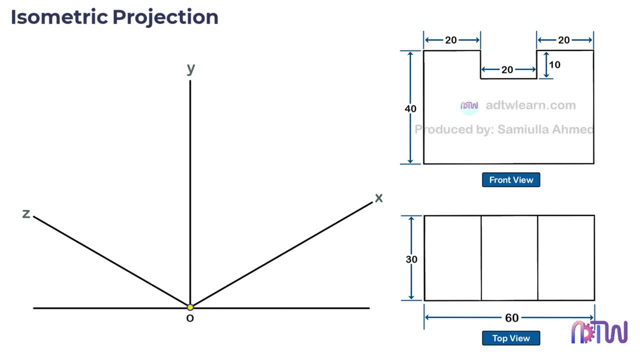 Let's first understand how this object looks in an isometric view. Consider this front view on this x-y plane. This is how it looks. By looking at the top view, we can see the front view is just extruded by 30 millimeters. This is how this object will look in an isometric view. This is 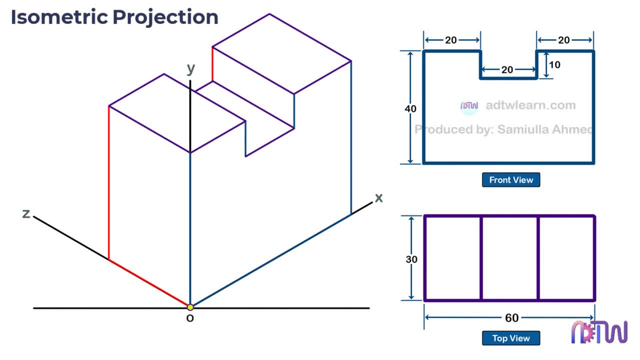 the front view and this is the top view which is given at the bottom. Let's start drawing. We will name the edges of this front view for our convenience: P, Q, R and S. Let's start drawing. We will draw the front view of the object facing on an x-y plane. 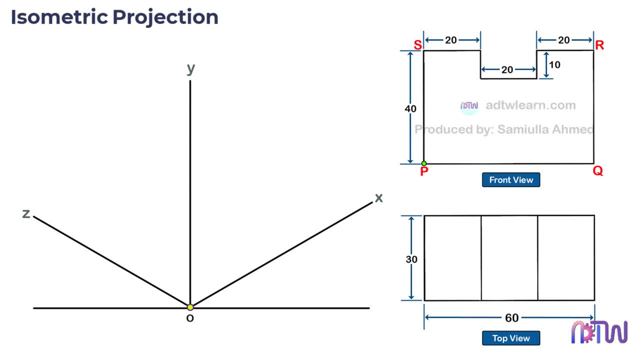 Therefore, while drawing, we will consider this left edge point of the figure as at this intersection point. Therefore, label this intersection point as P. Consider this x-y plane. On this plane we will draw the front view of this object. Initially, we will draw a rough. 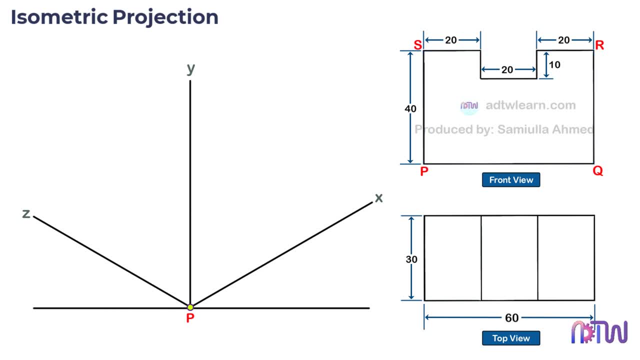 outline of this front view. on this plane We can see the height of this object in the front view is 40 millimeters. Take a roller scale and mark a point on the x-y plane. We will draw the front view on the y-axis at 40 millimeters. from the bottom We can see the total width of this object is 60. 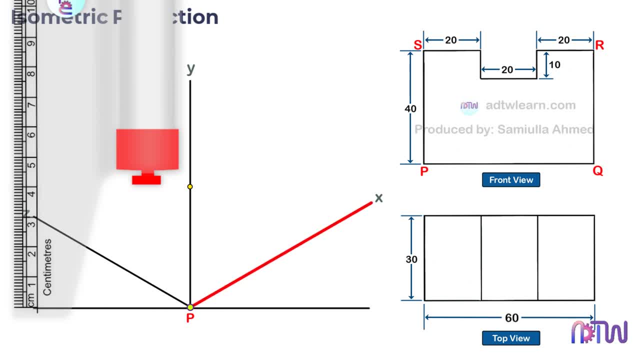 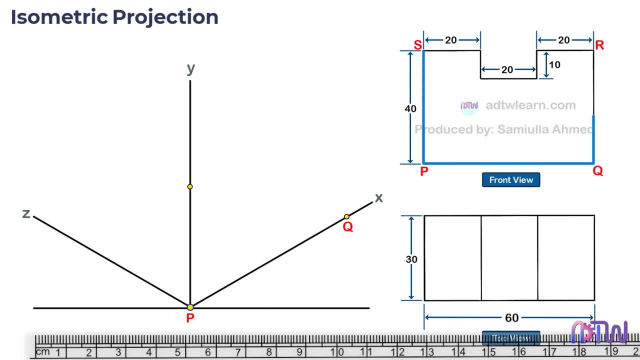 millimeters. Mark a point on this x-axis at 60 millimeters from point P. Label this point as Q. We can see this shape is a rectangle. Therefore, using the roller scale and taking this vertical line as a reference, draw a 40 millimeters vertical line from this point Q After this. 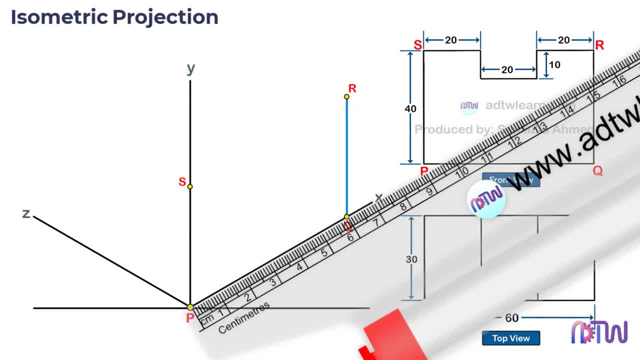 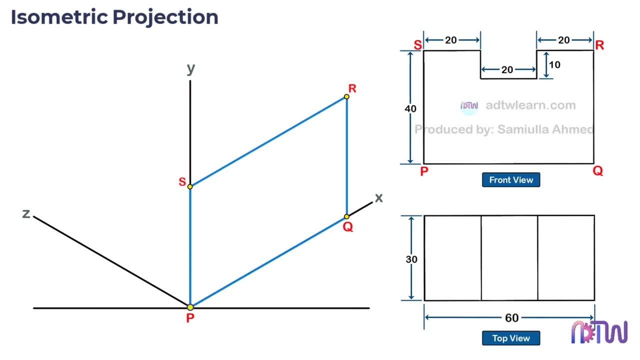 the x-axis is a reference. Join these points. This is only the outline of the front view on an x-y plane. After this we can draw the outline representing the top view. If we view the object from the top, then these S and R points will be here, So we will label these points as S. 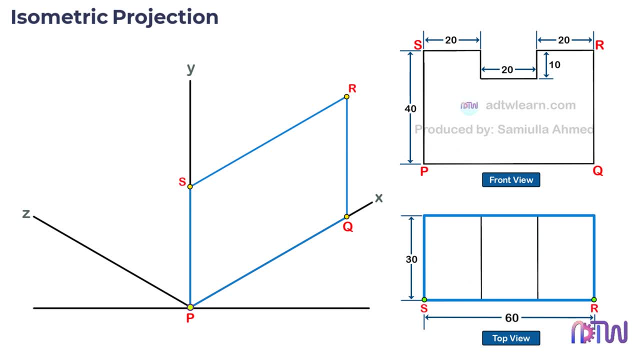 and R. We can see from this point S, the object length is 30 millimeters. That means from this point we need to draw a 30 millimeters line parallel to the z-axis. Draw another 30 millimeters line parallel to the z-axis from this point At the end, join these two points. This is the outline. 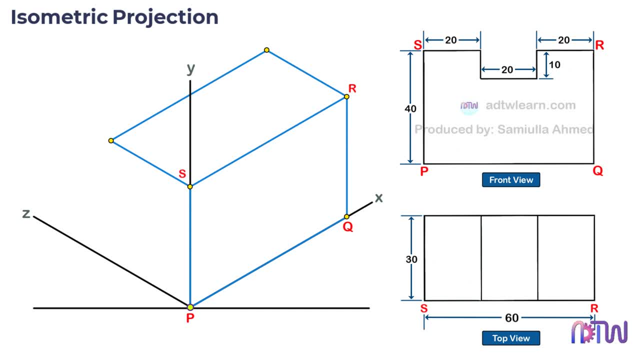 for the top view. After this, we will draw a vertical line of 40 millimeters from this point, since the object's height is 40 millimeters. After this join these endpoints, The height is 40 millimeters and the vertical line is 30 millimeters. This is the outline for the 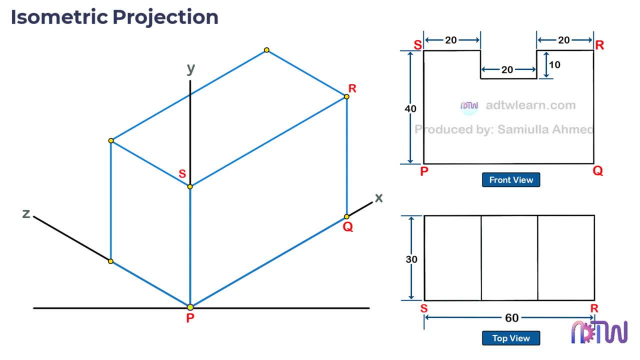 side view of the object. Since there is no side view of the object provided in orthographic projections, that means there are no additional details visible from the side view. Therefore, we can darken these lines, because this is how it will look at the end After this. 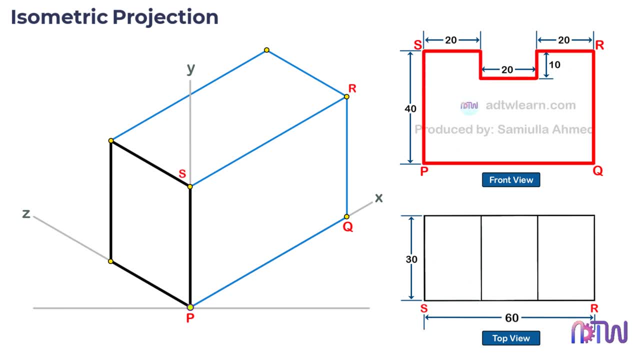 we can start drawing the details visible in the front view. We need to draw this slot on the front view plane. We can see the distance from point S is 20 millimeters. Therefore, draw a dark millimeters from point S. After this we can see there is a. 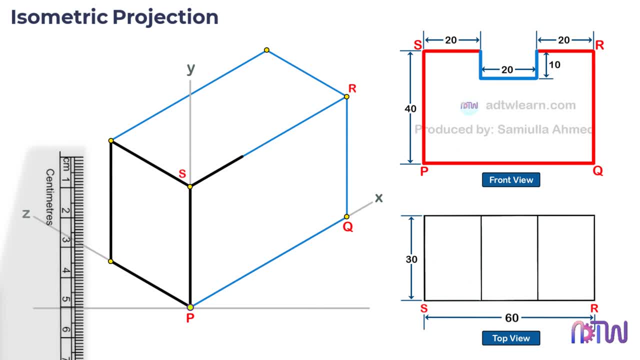 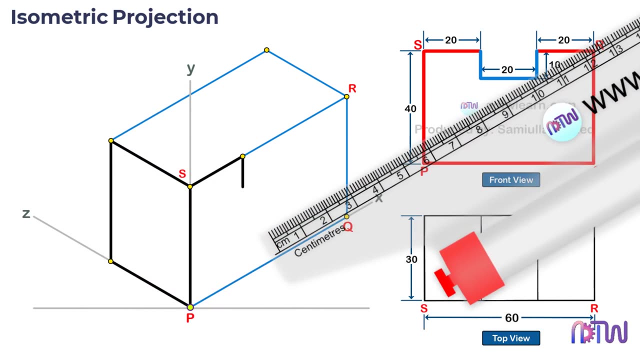 10 millimeters depth in this slot. Therefore, draw a 10 millimeters vertical line from this point. As we can see, the width of this slot is 20 millimeters. Therefore, draw a 20 millimeters line which is parallel to the X axis.